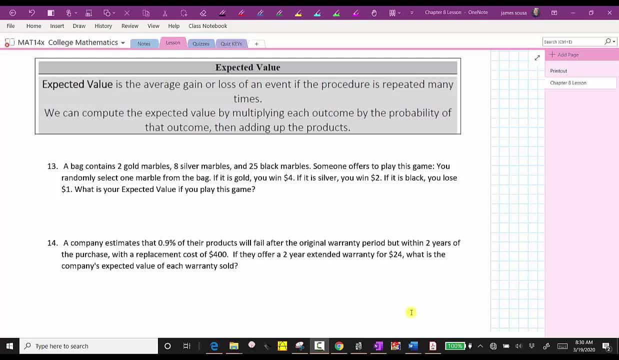 Let's take a look at two examples. For number 13,, a bag contains two gold marbles, eight silver marbles and 25 black marbles. Someone offers to play this game. You randomly select one marble from the bag. If it is gold, you win $4.. 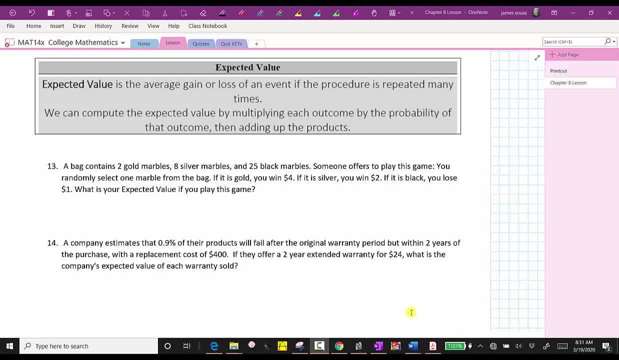 If it is silver, you win $2.. If it is black, you lose $1.. What is your expected value if you play the game? So the three outcomes are: you win $4, or you win $2,, or you lose $1. 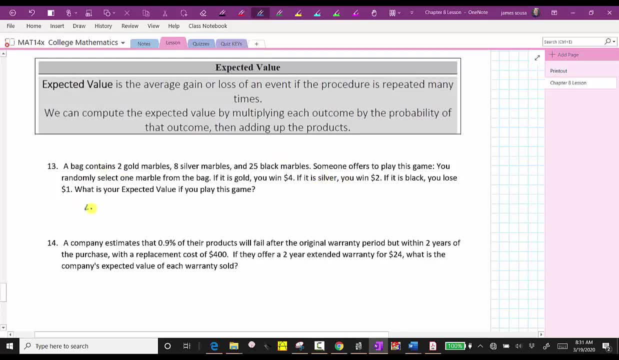 Let's begin with winning $4.. So we begin with positive four for $4.. Now we multiply this by the probability that you win $4, which is the probability of selecting a gold marble. Notice how there are two gold marbles out of a total of two plus eight plus 25,. 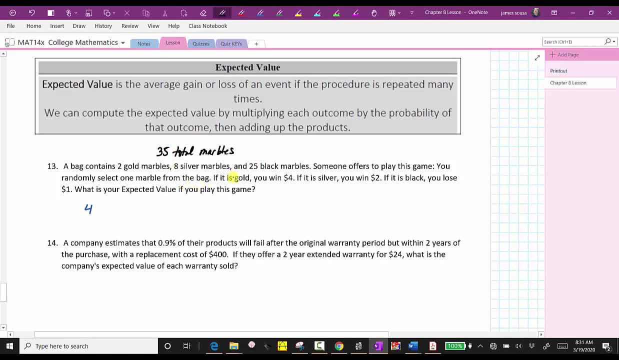 or 35 total marbles And therefore the probability of selecting a gold marble is two out of 35, or two divided by 35,, giving us four times two 35ths Plus, the next outcome is you win $2,. 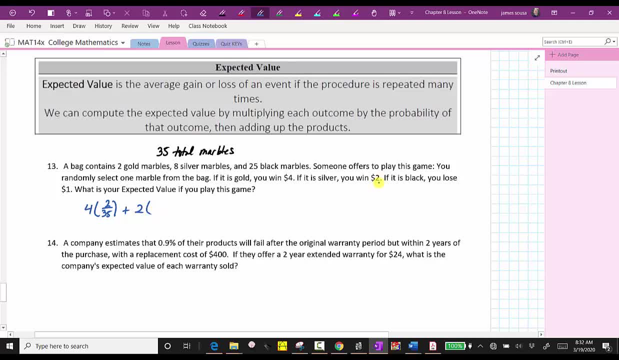 so plus positive: two times You win $2.. Of course, if you select a silver marble, the probability of selecting a silver marble is eight, 35ths or eight divided by 35. And then find the last outcome is you lose $1.. 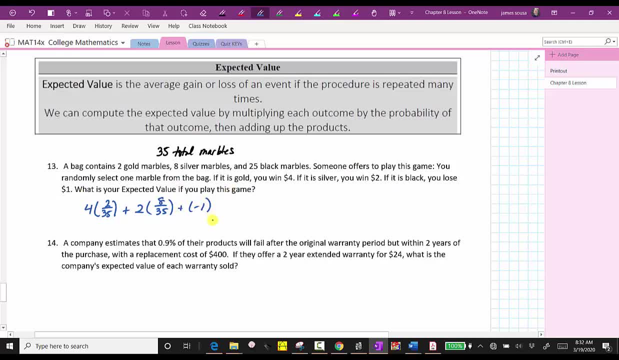 So we have plus negative one, because it's a loss of $1, times our probability of losing $1, which is the probability of selecting a black marble. There are 25 black marbles out of 35, giving us 25 divided by 35,. 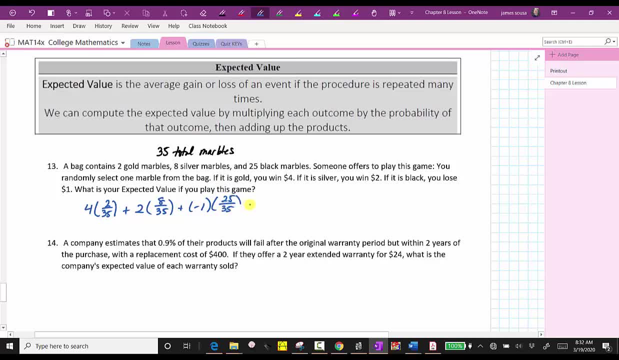 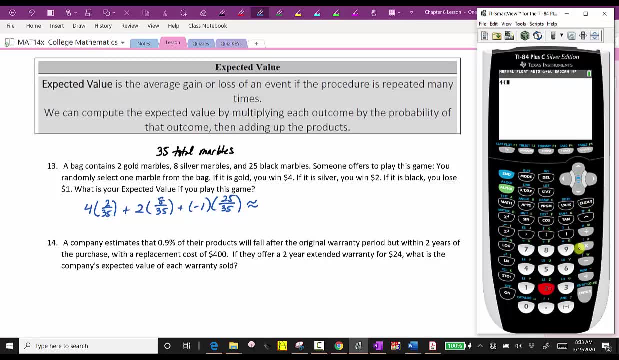 as the probability of selecting a black marble. The sum of these products will give us the expected value. Going to the calculator, we have four times two divided by 35, plus two times eight divided by 35. And then we can write plus negative, one times 25, 35ths. 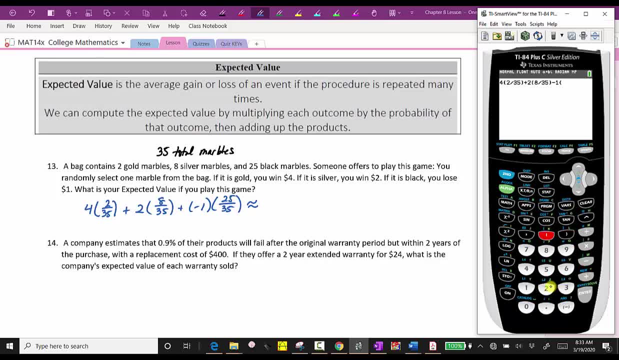 or just minus one times 25 divided by 35. And this is in dollars and therefore we round to the nearest cent, which gives us negative 0.03, because we have an eight in the third decimal place. So the expected value is negative $0.03,. 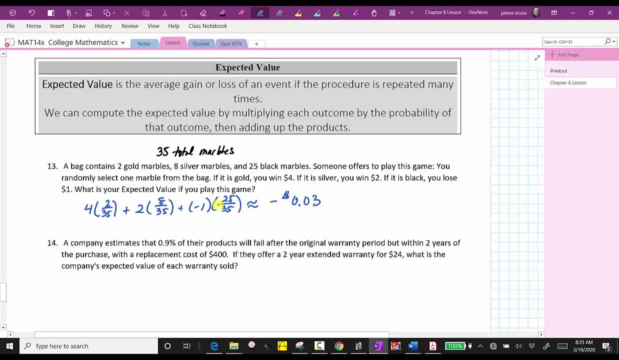 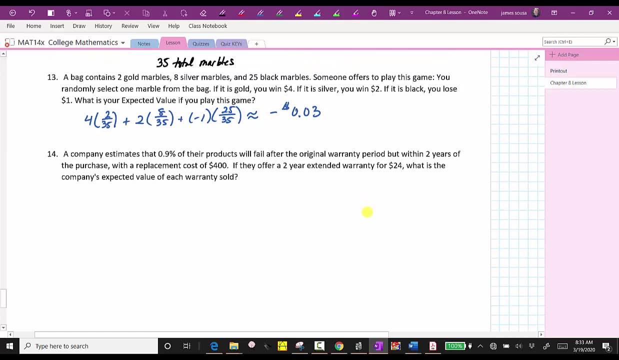 or negative three cents, which means, as this game is repeated many, many times, the average loss is going to be three cents each time it's played. And now let's take a look at number 14.. The company estimates that 0.9% of their products will fail. after the original warranty period, but within two years of the purchase, with a replacement cost of $400.. If they offer a two-year extended warranty for $24,, what is the company's expected value of each warranty sold? So the first thing to recognize here: 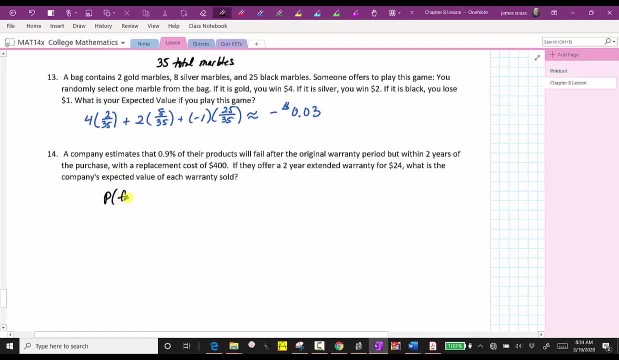 is the probability the product will fail. The probability of failure is equal to 0.9%, which must be expressed as a decimal, which is 0.009, which means the probability of no failure is equal to one minus the probability of failure. 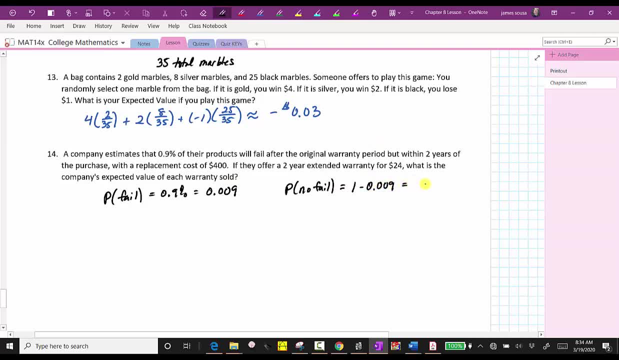 which is one minus 0.009, which is equal to 0.991.. We need both of these probabilities to determine the expected value. Now, one outcome is the product fails and the company has to replace the product at a cost of $400. if they don't lose all that money. 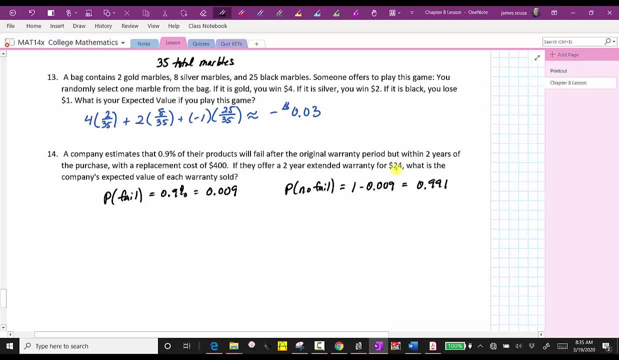 because the customer would have had to purchase the warranty for $24.. So if the product fails, the outcome is negative 400 plus 24.. The negative 400 is the cost they have to pay to replace the product, but they do get $24 because the customer did purchase. 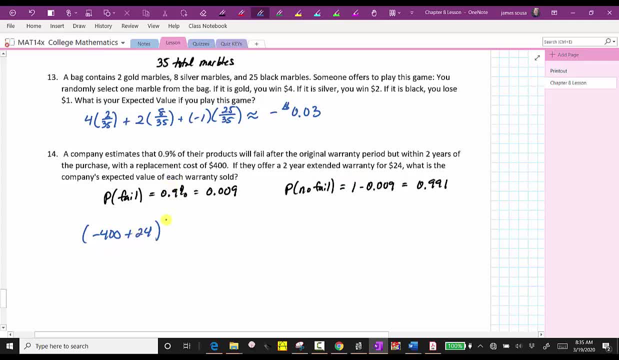 the warranty. So this is the outcome if the product fails, and then we multiply this by the probability of failure, which is 0.009 plus, the second outcome would be: the product does not fail and therefore the company does receive the warranty cost of $24,. 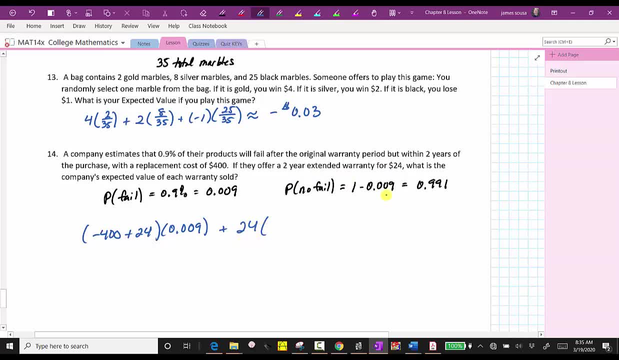 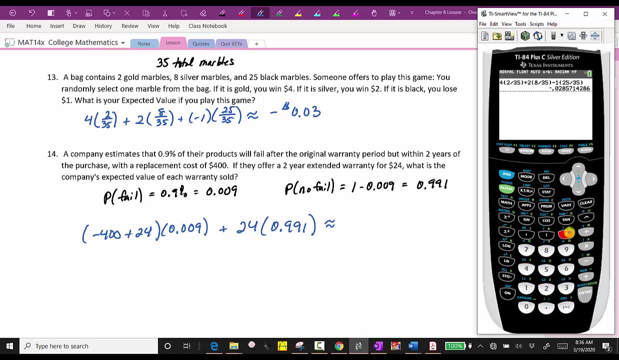 which would be plus 24 times the probability of no failure, which is 0.991.. And now we go back to the calculator and round to the nearest cent, We have negative 400 plus 24- in parentheses- times, 0.009,.